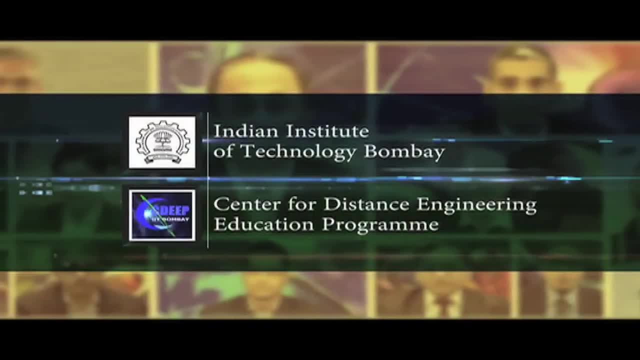 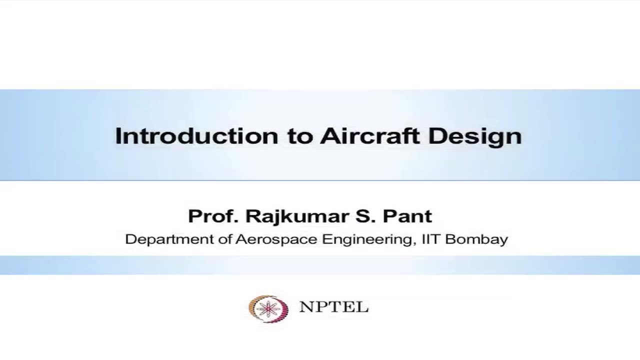 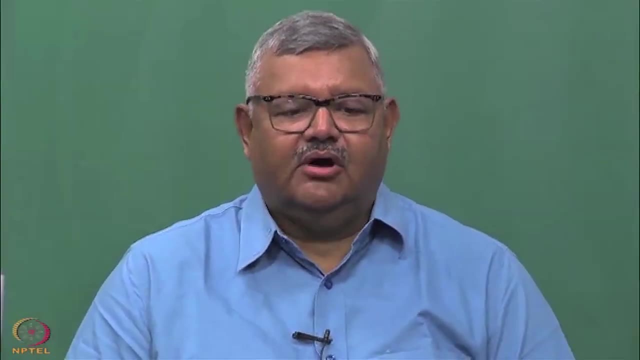 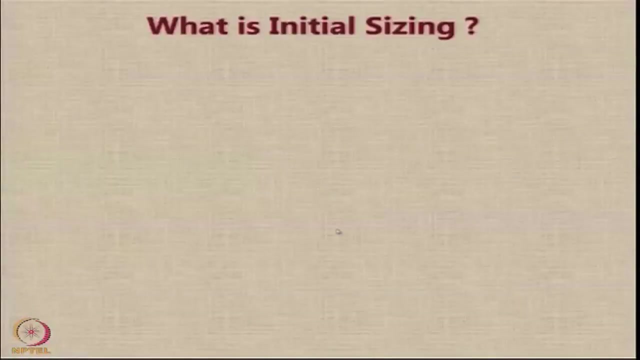 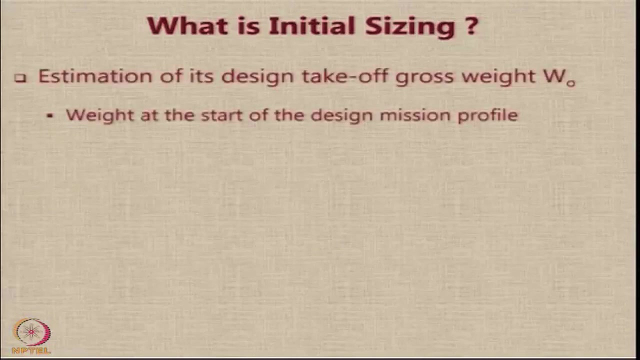 Alright, let us look at the concept of initial sizing in aircraft design. This is the first step in design where we start looking at some estimates or some numbers. What is initial sizing? The words initial sizing in aircraft design have a very specific meaning and that 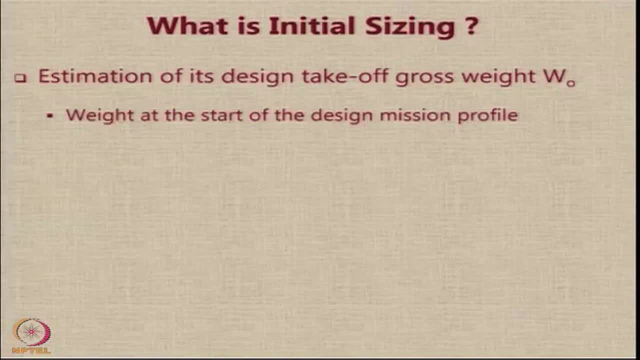 meaning is estimation of the aircraft design takeoff gross weight. Now, what is design takeoff gross weight? It is the weight of the aircraft at the start of the design mission profile. Every aircraft is designed to meet or to operate its mission using a specific 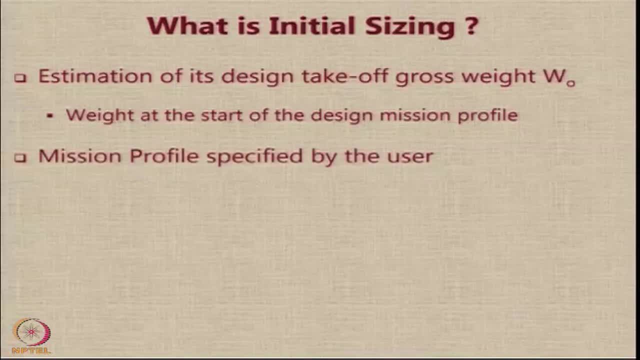 profile. This mission profile is essentially a sketch that indicates what the aircraft is supposed to do, And this is specified by the user. But apart from the mission profile given by the user, there are some additions, Additional requirements, which also have to be taken care while carrying out the sizing. 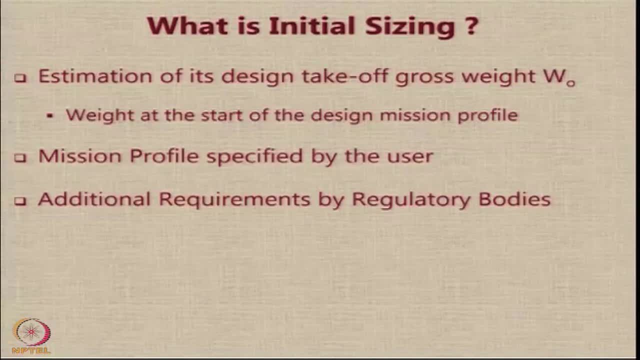 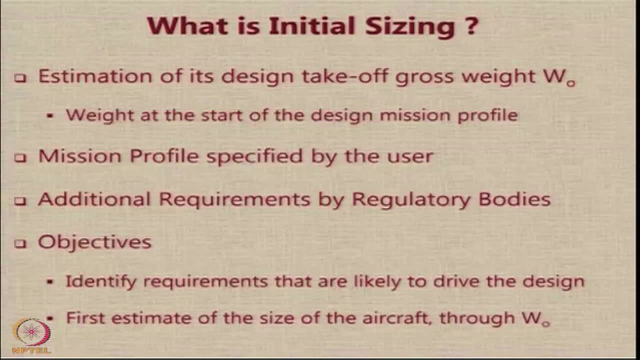 These requirements, as we know, are specified by the regulatory bodies. So the objective of initial sizing are twofold: First is to identify the requirements that are likely to derive the design And, secondly, to get a first estimate of the size of the aircraft. 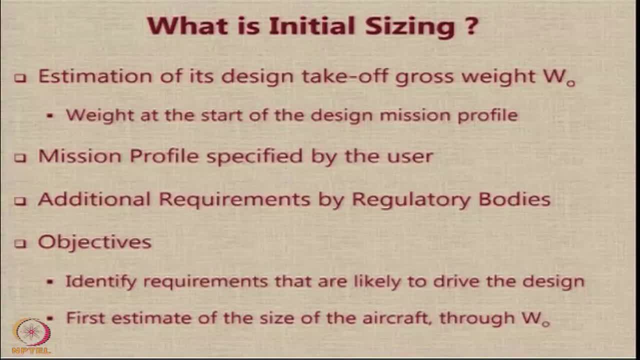 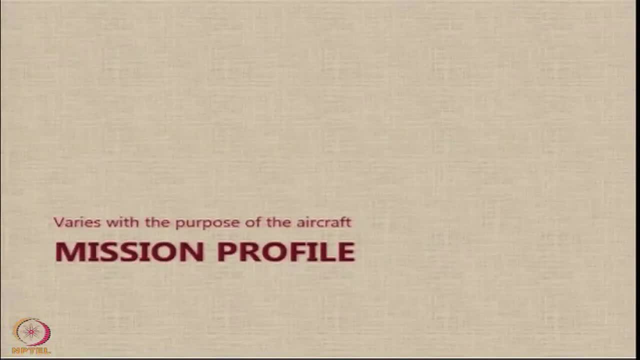 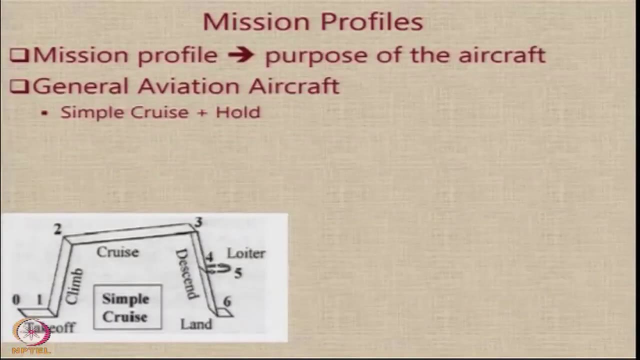 through the estimation of its design. Mission profile is something that varies with the purpose of the aircraft, So let us have a look at some standard mission profile Now. if you have a simple general aviation aircraft, then the mission profile is very straightforward: You just take off, climb to the height, cruise. 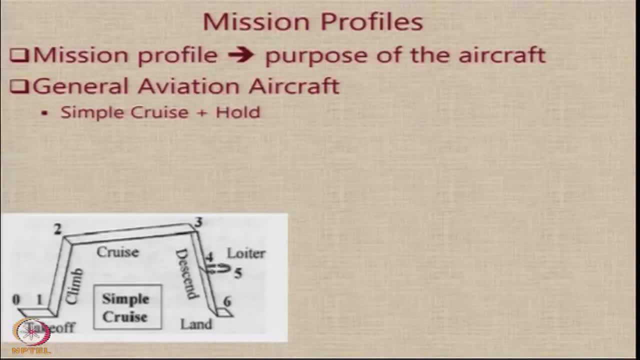 descend descent. you may be forced to loiter for some time because the runway is not available to you. This requirement of loiter is normally specified by the airworthiness agencies. we call it as a hold And then, once you are cleared to land, you would be then proceeding with the descent. 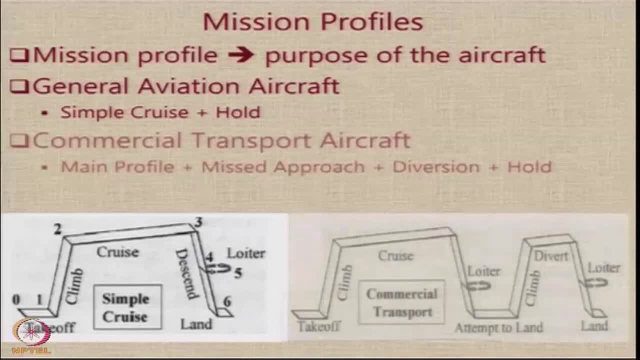 and landing. When you have a commercial transport aircraft, the mission profile is slightly more complicated. Apart from the initial profile, which is similar to the general aviation aircraft, you have to also keep a provision for one attempt to land which is unsuccessful, And this could be because of a various of reasons. it could be because, when you are 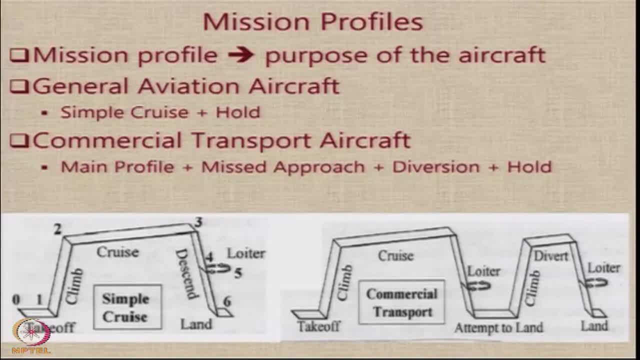 attempting to land there is some obstruction on the runway, or, when you are attempting to land because of weather or any other reason, you are forced to abort the landing and divert to A nearby airport. So you should have enough fuel to be able to climb after an attempted landing, which 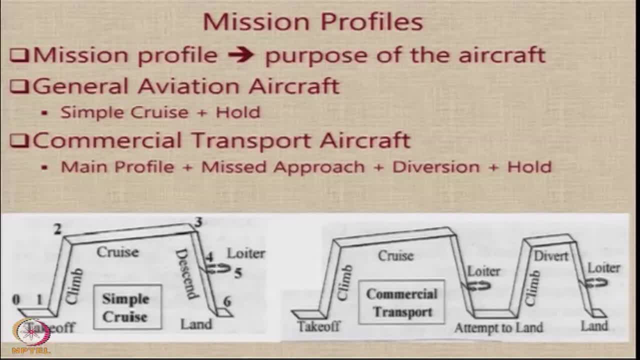 is aborted, divert to a nearby location, approach and again have some fuel for loiter, because even at that airport you may have to hold for some time and then land. So these requirements for loiter and diversion and the second loiter are the requirements. 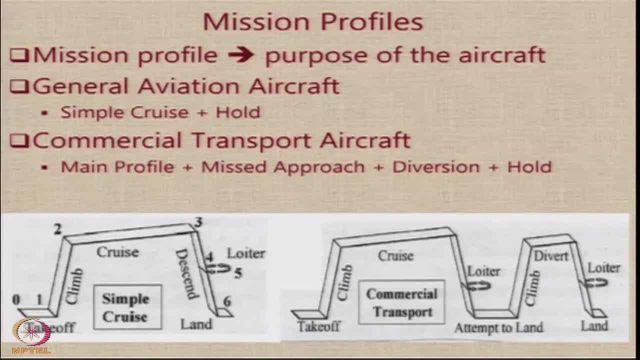 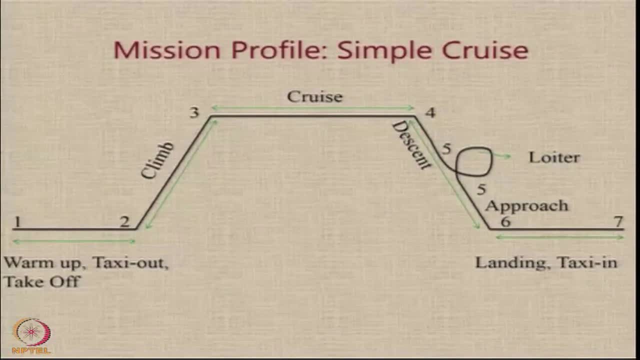 which are given by the airworthiness agencies, Essentially to ensure our safety. Let us have a look at a simple cruise. The mission profile of a simple cruise can be broken down into various subsegments. So, for instance, you have the first leg, which is the warm up taxi out and take off. 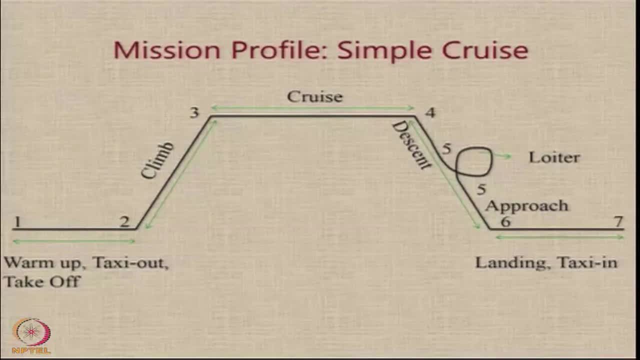 Every aircraft spends some time in. the pilot need some time to check all the systems just before the takeoff is commenced. Typically, the pilot would pull the put the aircraft, would start the aircraft and go for a checklist, and during that time the engine is on and hence fuel is being consumed. 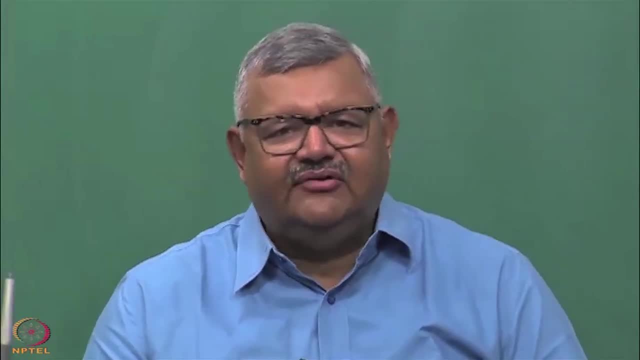 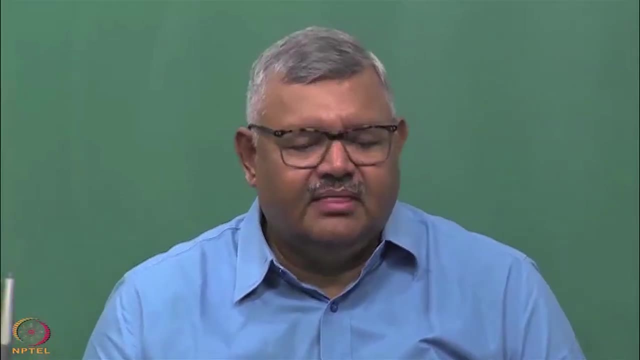 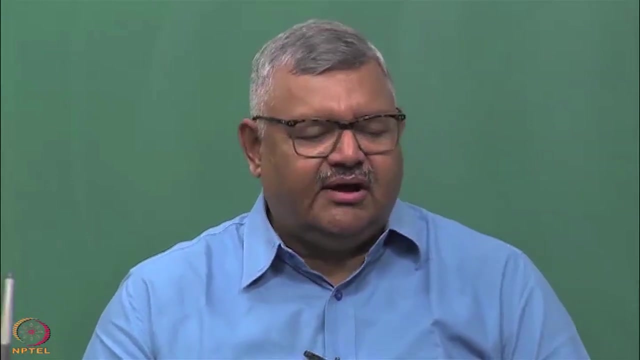 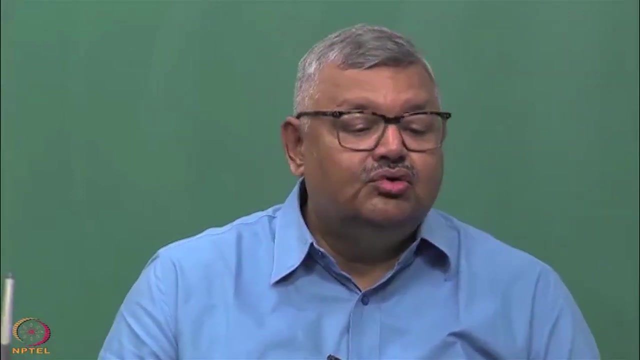 After that, once you are given the clearance to proceed, you have to taxi out, that is, to proceed from the place where you are parked, or the terminal or the gate, to the start of the runway and then from there you have to execute a takeoff. So during this phase, when you are still on the ground, in many ways you are going to consume. 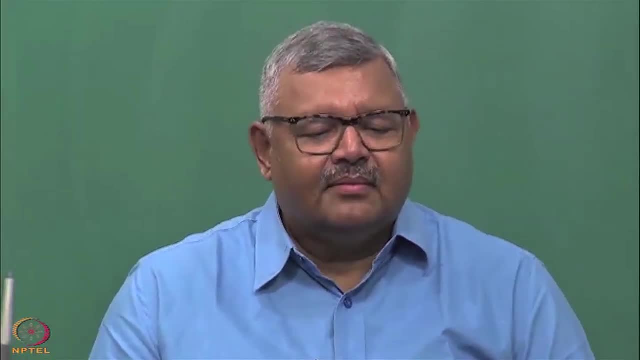 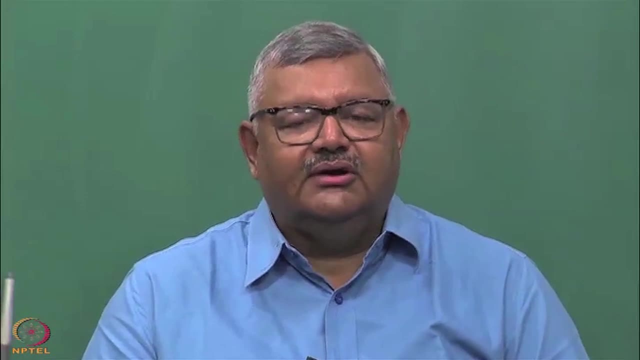 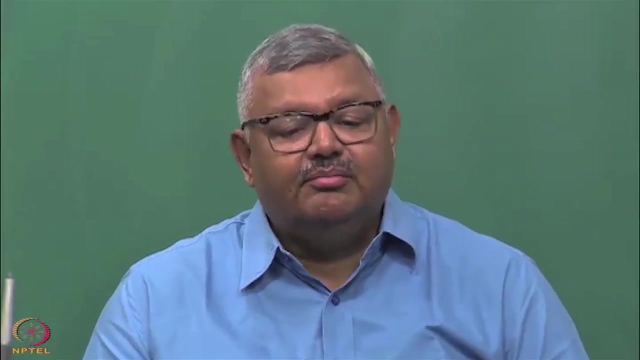 some amount of fuel. therefore, this is the first leg. the second segment would involve climb to the cruising altitude. The next would involve cruise to the runway To the desired destination. This cruise could be a constant altitude cruise, as shown here, or it could be a cruise climb. 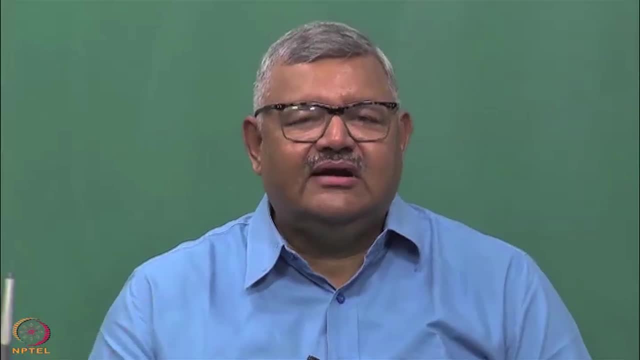 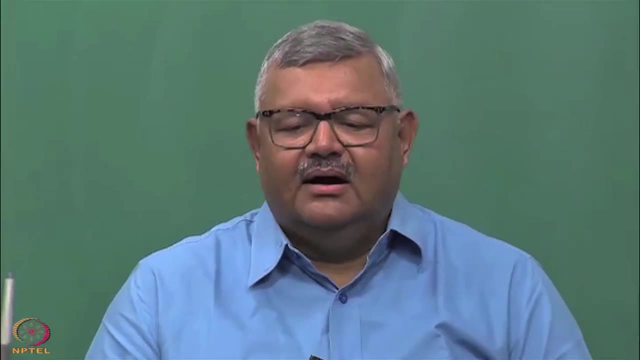 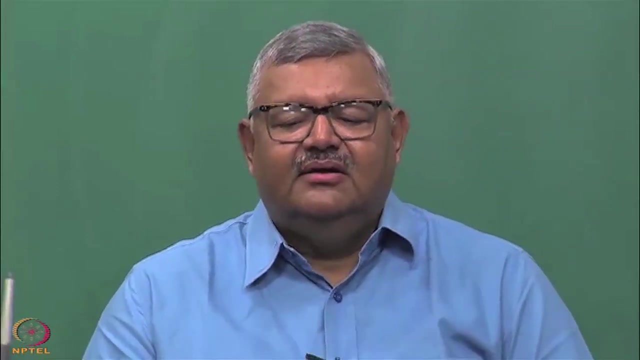 in which the altitude is constantly increasing because of consumption of fuel. that is a matter of detail, so that is not shown here- And then you have a descent phase, when you are now approaching, when you are wanting to now land, but when you are descending you might have to actually go for some amount of light. 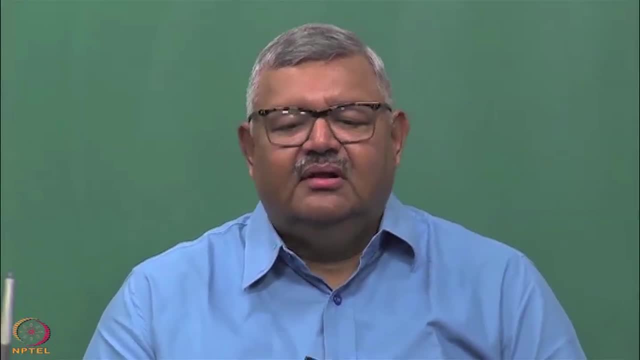 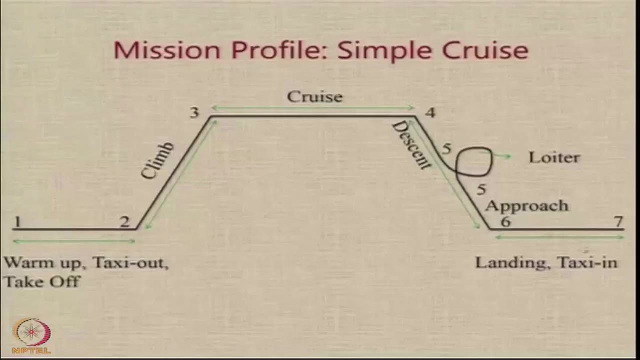 or hold at the destination airport and then, once you are cleared to land, you will have a approach segment and then you will have the landing segment. After landing, you are going to taxi into the terminal or the gate once again. So each leg of the mission profile is assumed to start and end from numbers. for example, 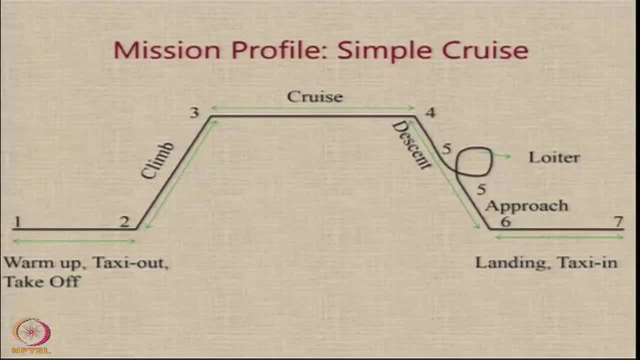 the warm up, taxi out and take off is from 1 to 2.. So the leg is 1 to 2,, 2 to 3, 3 to 4,, 4 to 5, 5 to 6,, 6 to 7.. 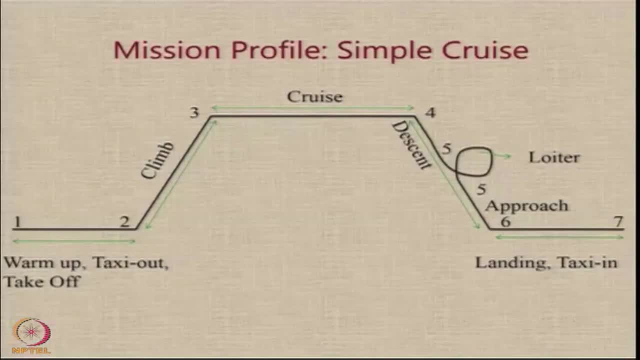 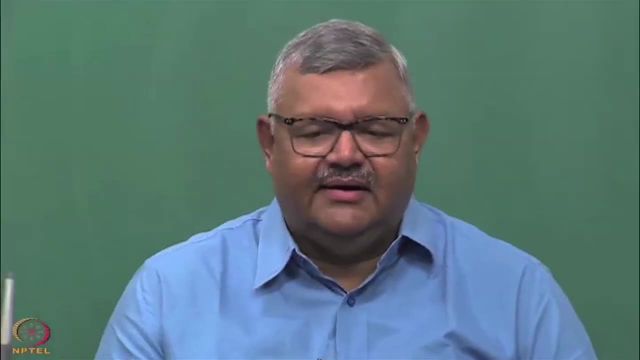 Now, if it is a transport aircraft, as you know, after this there will be a requirement for between, between approach, there will be a, and land, there will be a requirement for diversion, which will involve another climb, another small cruise, another descent, another loiter and then final landing in. 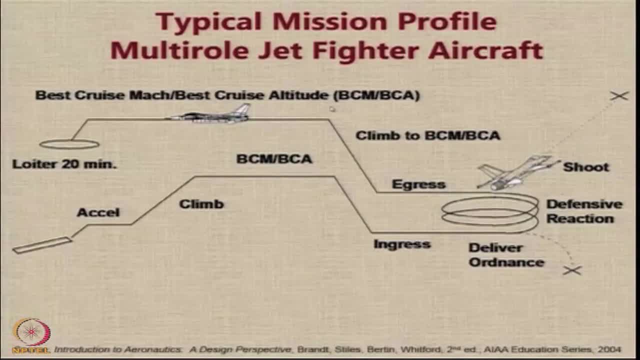 This is a typical mission profile for a multi-role jet fighter aircraft. Here you take off, accelerate, climb and then you fly out at the best cruise mark number and the best cruise altitude. Notice, the requirement is not specific here. You are allowed to choose and then, when you are going to reach the area of operation, you 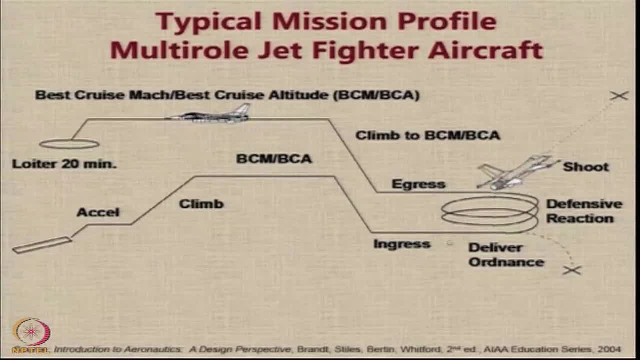 are going to come down to the low altitude, there will be an ingress. at the combat erosion, there will be delivery of some ordination And then you have to avoid. you will have to have some defensive reaction. After that, once your job is over, you are going to egress back again. you will climb to a best 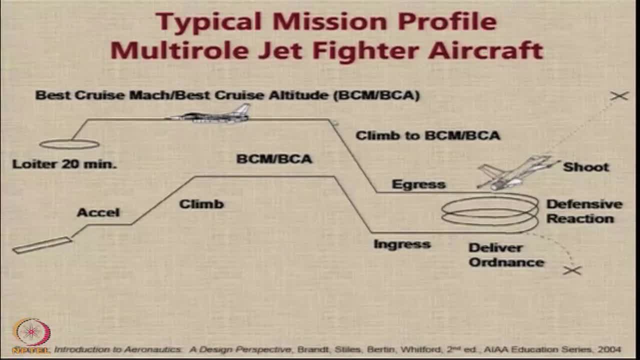 cruise altitude at best cruise mark number, and then you continue your flight back to the origin and when you come back you may have to loiter for some time. So this is a typical mission profile for a multi-role jet fighter aircraft like that. there are many mission profiles which have to be considered. 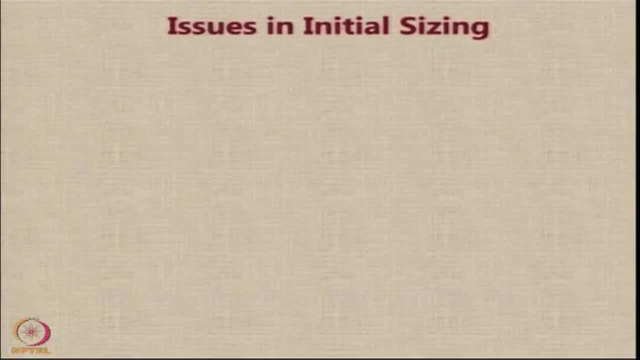 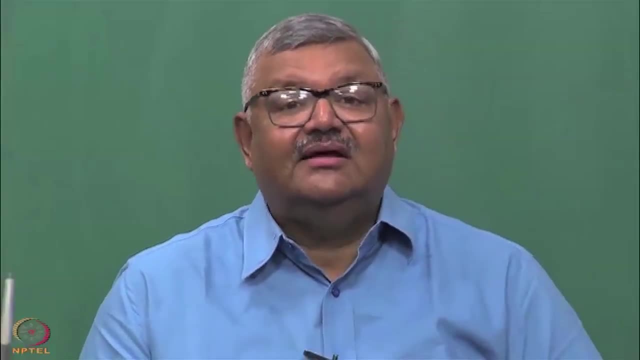 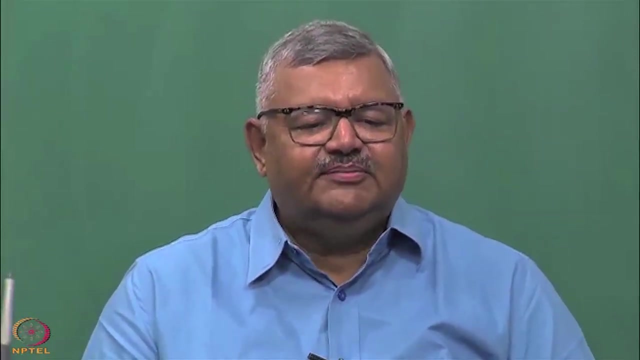 In our in our explanation, we are going to focus only on a civil transport aircraft. Now, right in the beginning, it is important for us to realize that there are some fundamental issues that are going to plague us when we do initial sizing. The first problem is that you would like to estimate the gross weight of the aircraft. 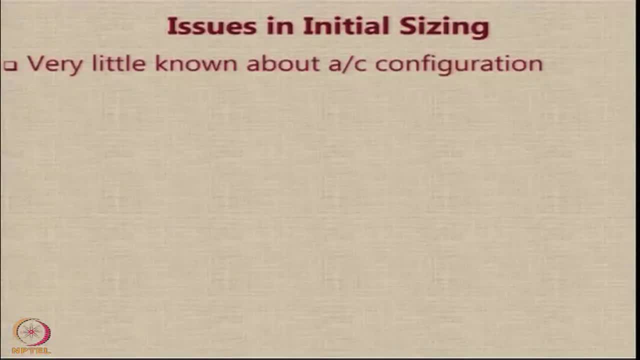 but you have very little information about the aircraft configuration. you have not yet designed the aircraft. You have not even arrived at what kind of shape or configuration you will use. All you know, probably, is that this will be a turbofan engine aircraft which will have 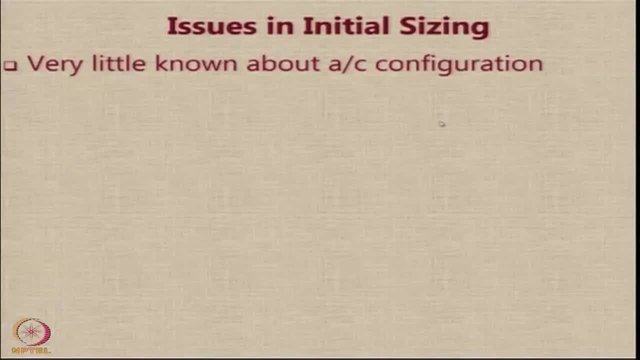 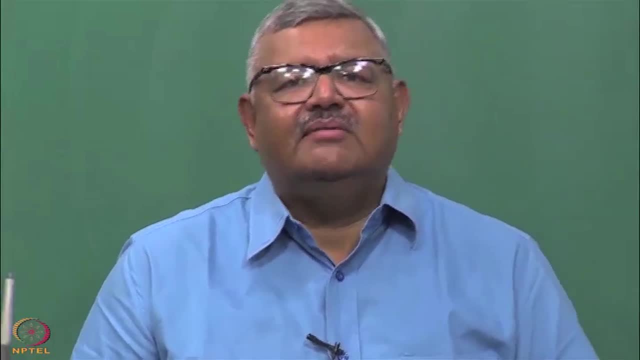 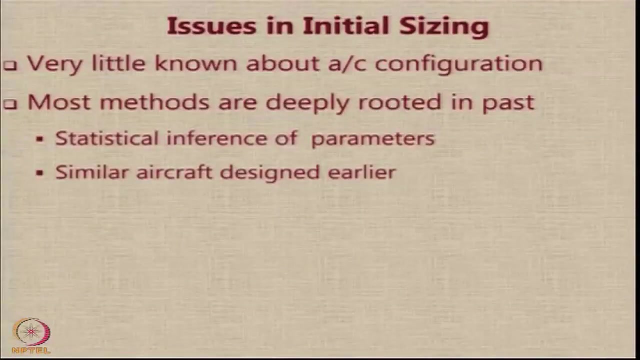 in the typically this kind of you know configuration. you do not have the specific configuration yet, you only have a very vague idea, but with very little information you are supposed to do estimates. So therefore, Most of the methods that you will see in the initial sizing are very deeply rooted in the 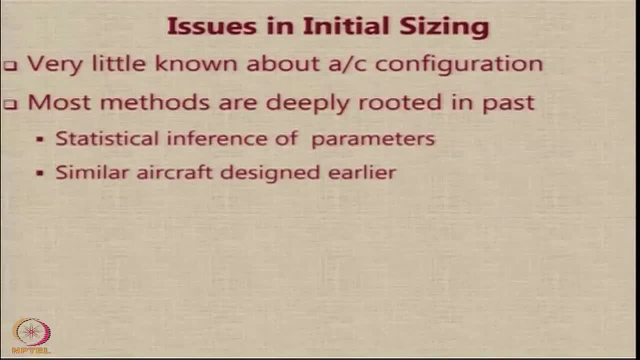 past. Most of the formulae and procedures are going to be basically extrapolations or interpolations within the database available for the existing aircraft. The estimates are going to be arrived by statistical inference of the parameters and it will be based on the data that you have collected. 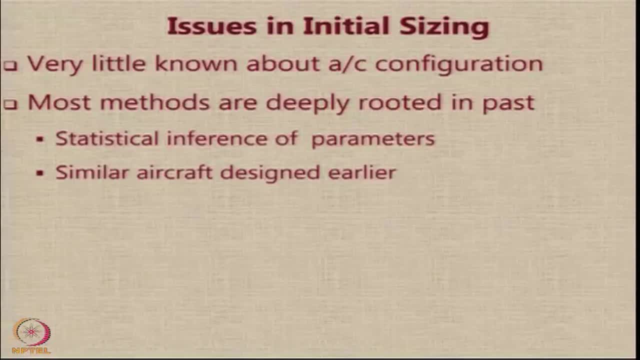 For Similar aircraft which are designed earlier, and this is why most aircraft designers they have with them a large database of information regarding the existing and the past aircraft. Okay, Because you are going to now make an estimate without great information about your aircraft, without much information about your aircraft. 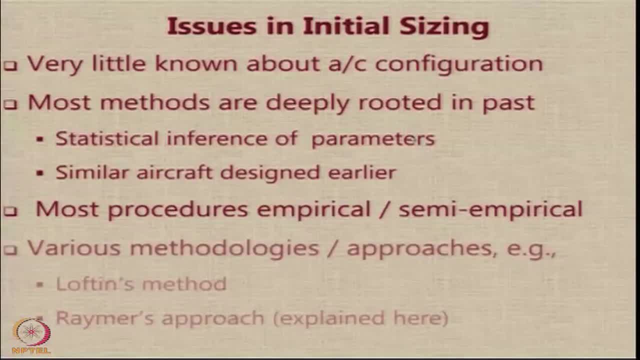 So therefore, you have to go for empirical and semi-empirical procedures. Now, In literature, There are many, many methods available for carrying out initial sizing. One of the methods which was quite popular earlier, was given by Lawrence K Loftin Jr.